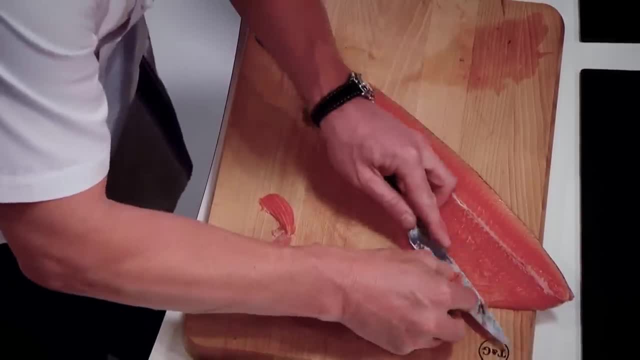 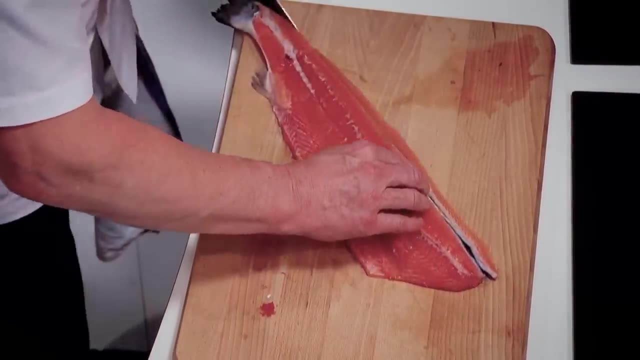 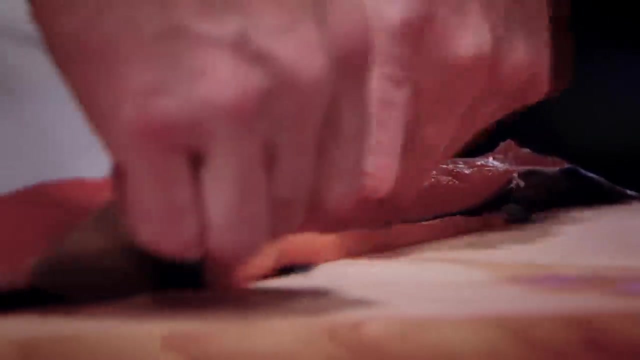 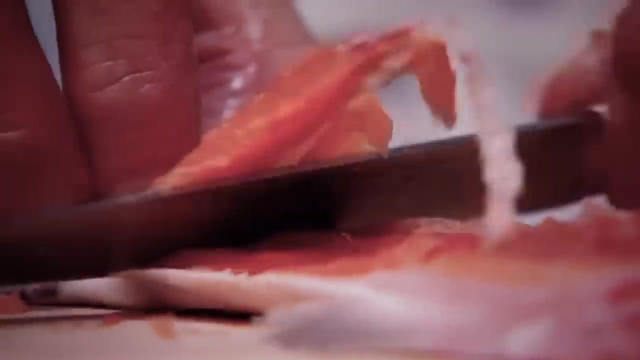 that's where that flavor is. Again, clean board, clean knife- you've got clean slices. Use the sharp knife, Come through, slice down through the dorsal fin and remove that off. You can see there's a bit of bone left on there. Come back up in and off There, Remove the fin. 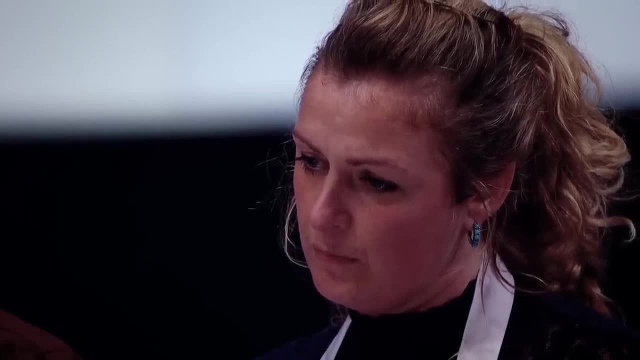 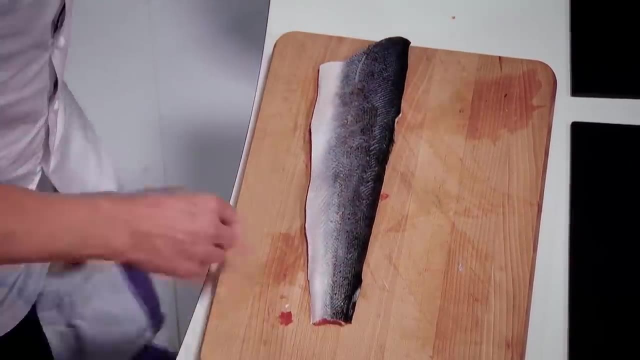 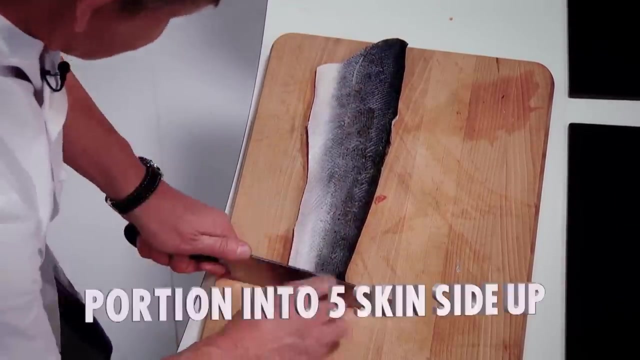 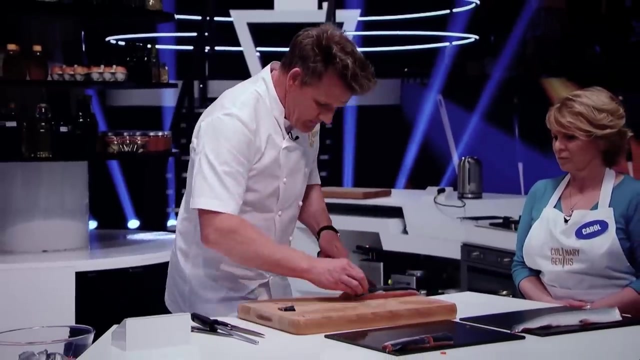 Very carefully. Every time you do this you're taking off minimal cuts of salmon for obvious reasons. Turn that over. and then think about the portions One, two, three, four, five. So we trim the tail There. One, two On Three. 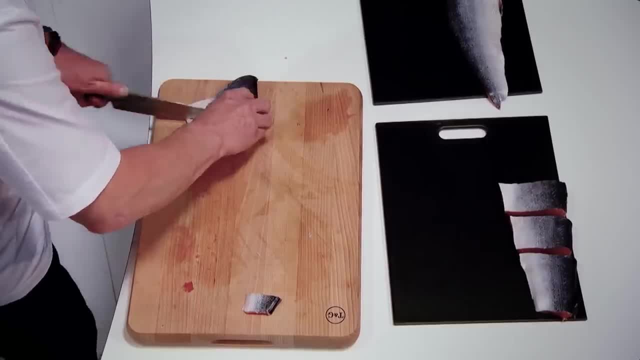 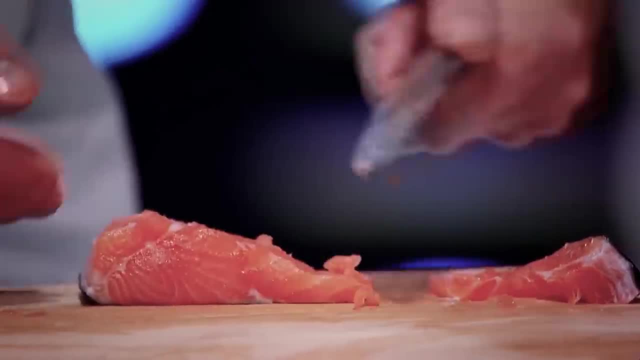 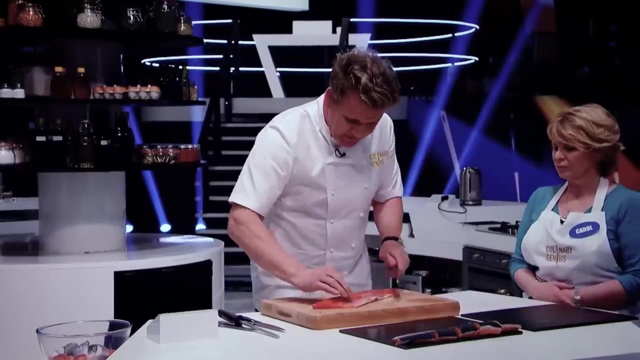 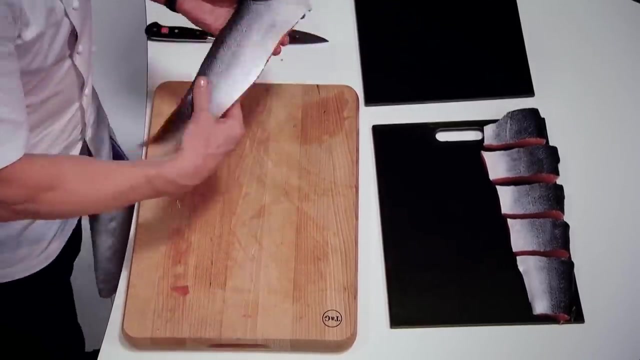 Four On, And this bit here just tidy that up a little bit. Five On Second side: Clean the board down. Same procedure again: Big knife round the fin. come off Nowhere near as many bones this time around. Turn it around, Look at the cut Mirror. what you've just done there. 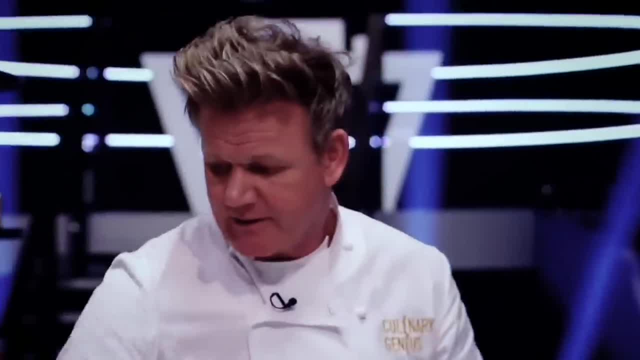 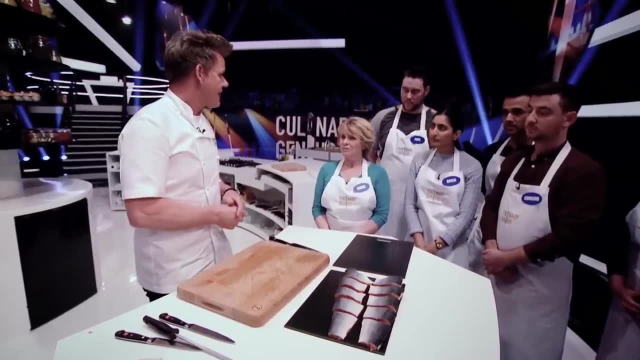 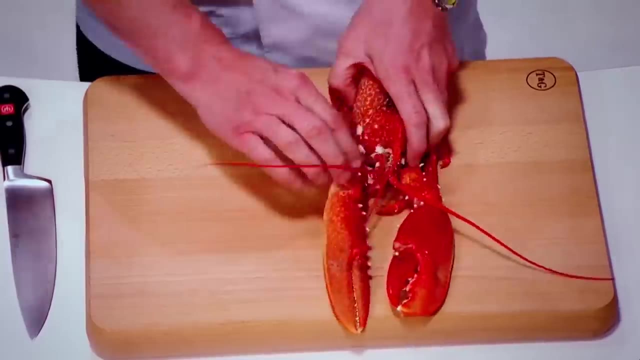 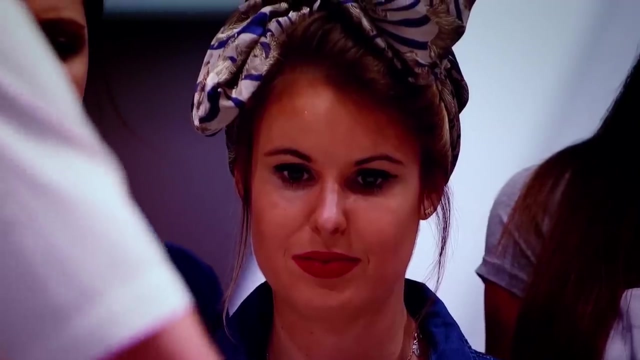 And there we have two, four, six, eight, ten portions of salmon filleted Lines with precision and finesse. Ten portions out of your salmon, Understood? Sure, Yeah Right. Lobster First off, off with the claws. Now, from there, tail lift open and twist Okay. 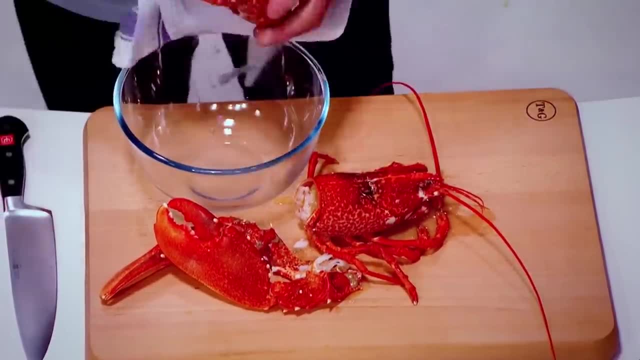 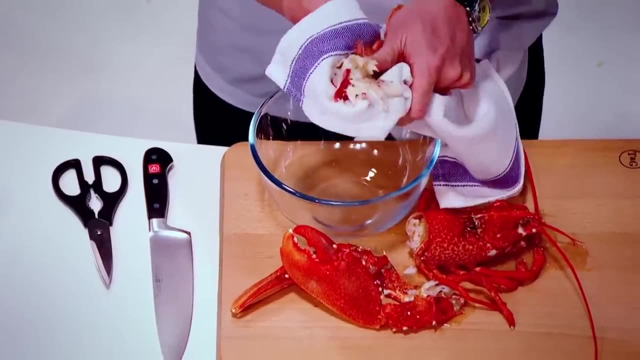 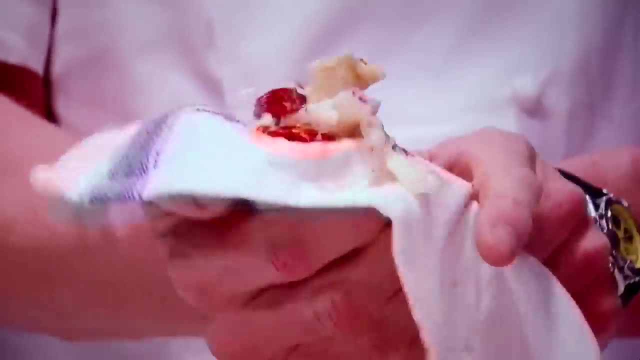 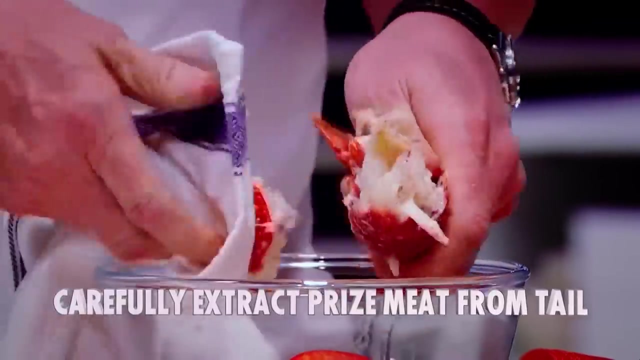 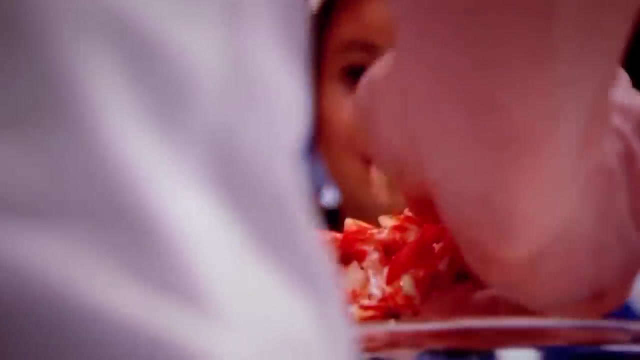 Now open. Open up that tail, Press it in between your hand, palm of hand, in and squeeze the top part of that tail, Literally squeeze. Once it's squeezed, hold it open and twist And literally do not burst the lobster. And then, when you get down to the third one thumb on here, push in and 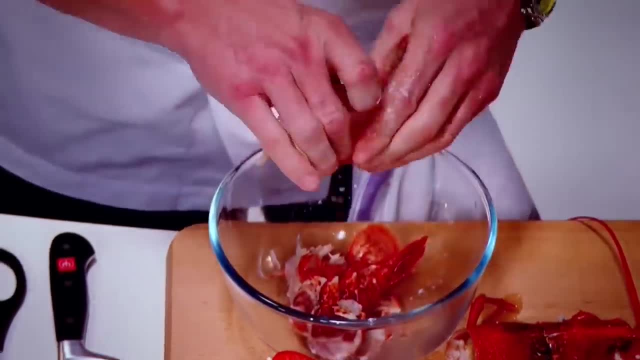 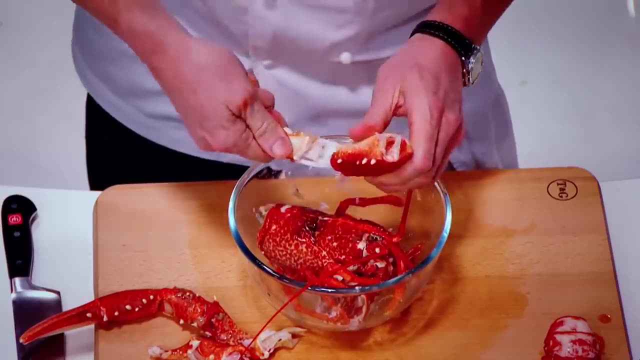 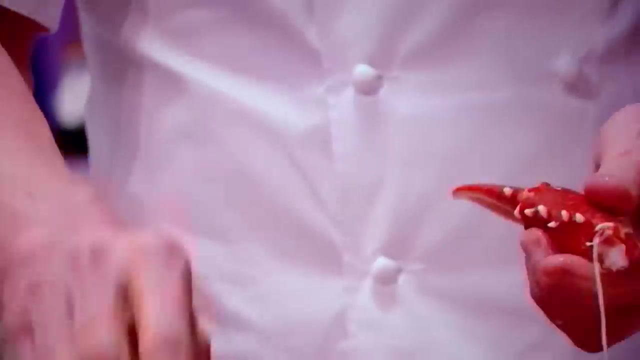 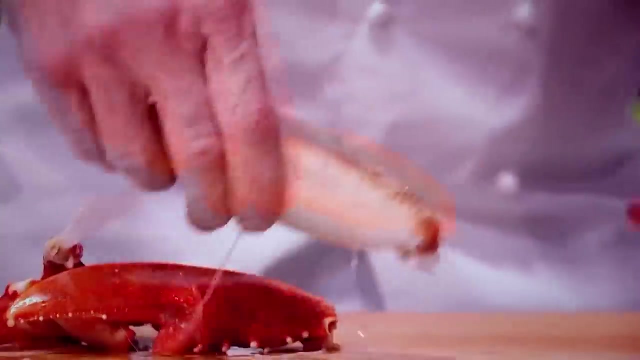 gently, literally pull out the tail From there claws. separate the knuckle, pull the first claw, twist and pull, Turn it out, Get rid of that water Again, separate the knuckle, twist, Drain out and pull From there big knife, Hold up the claw In. 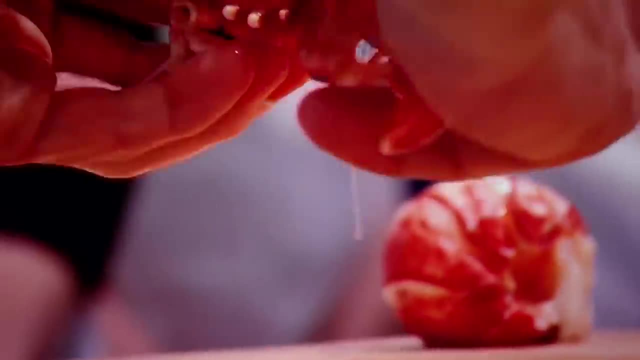 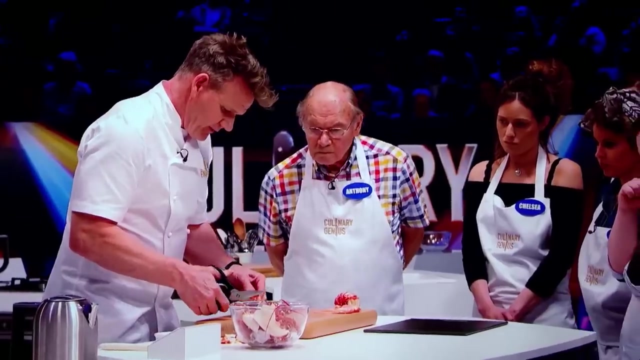 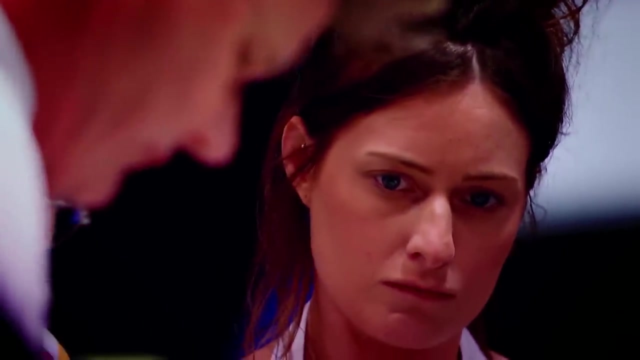 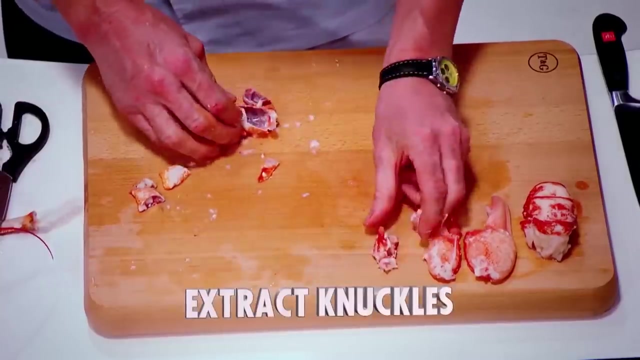 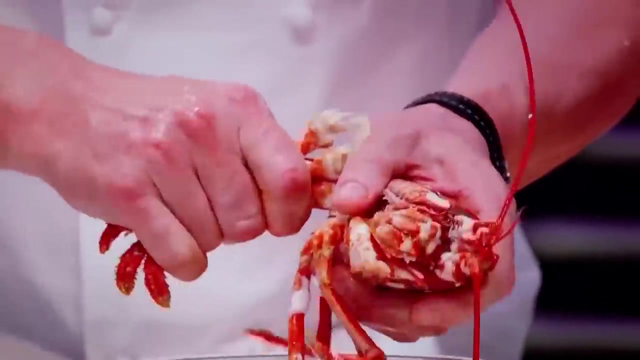 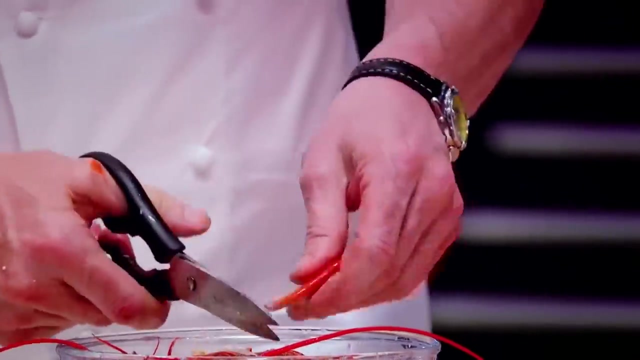 Twist, Burst off little finger in off with the claw. knuckles off there through here. slice one half down, push from there, open up. beautiful. okay, one knuckle out First. take this off. These little beauties have a touch of meat. I'll show you where These bits here top. try and slice at an angle, Rolling pin at the back, push and out comes the leg. 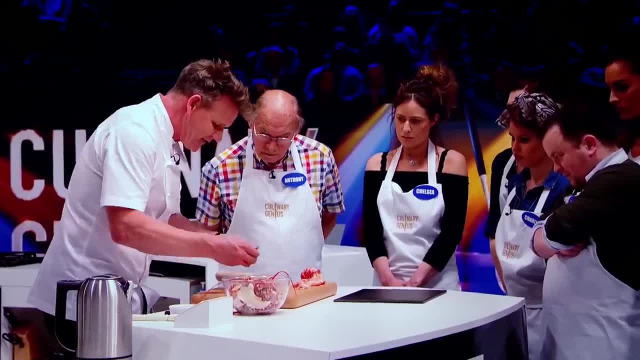 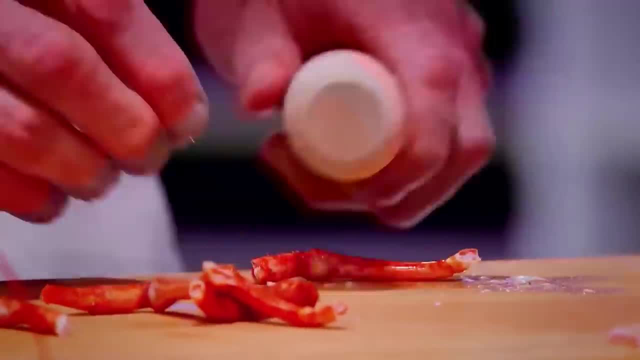 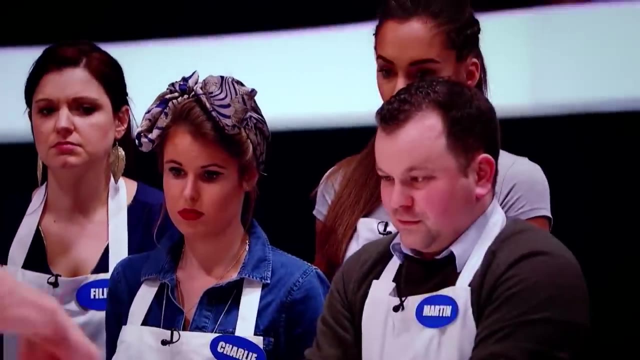 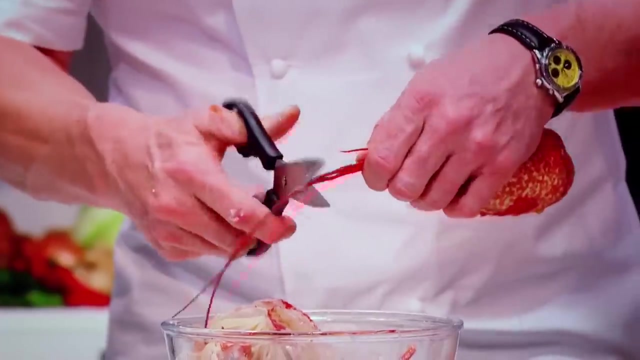 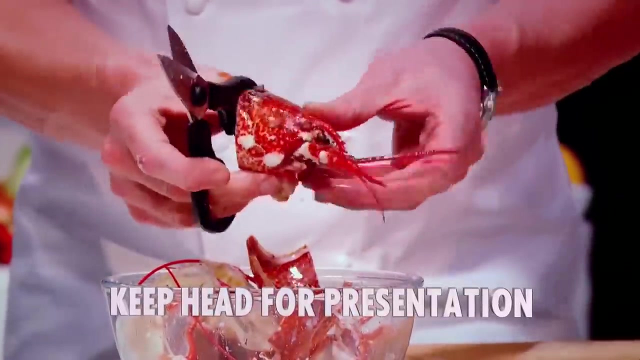 These are tiny little legs, but the meat inside is so sweet, It's extraordinary. Again, slice at an angle, open up the knuckle, Take this off Down in and squeeze From there. take the head, cut tentacles off. There's a V here. Go round, present your lobster, Take out that. 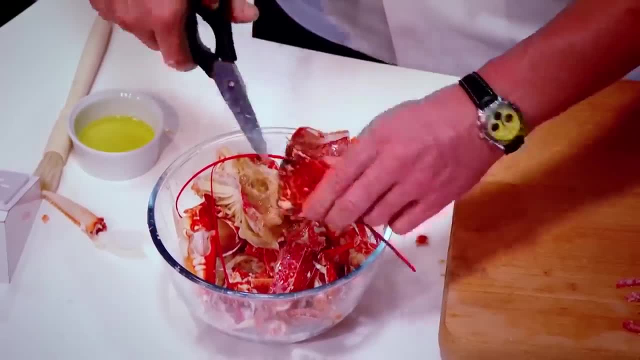 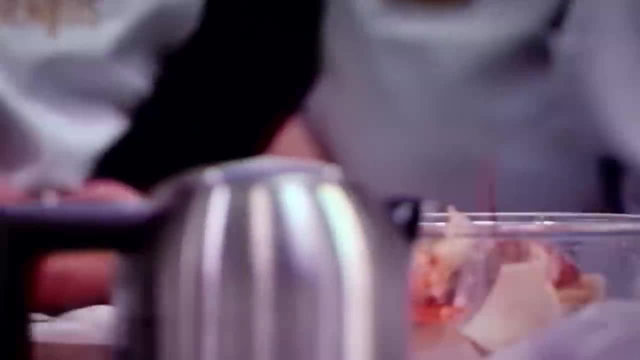 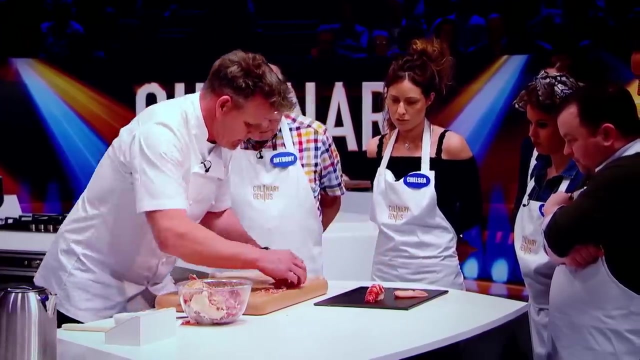 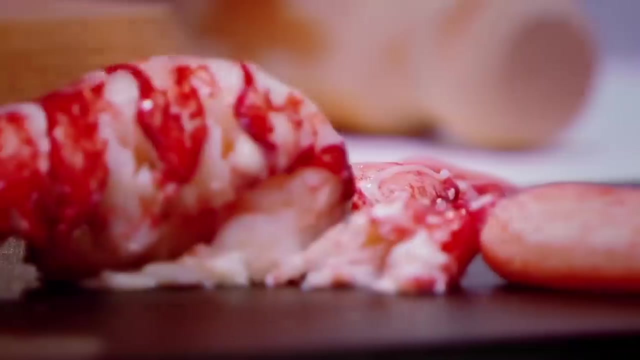 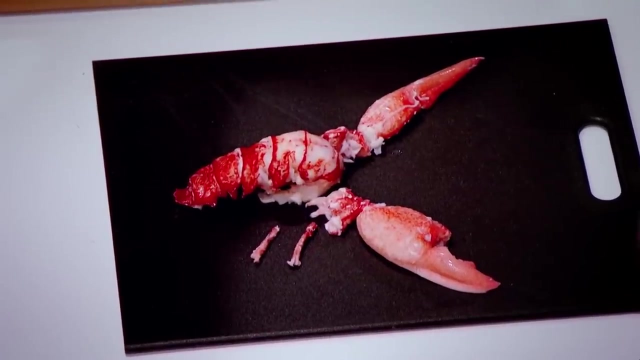 Now, that's just a touch of the carcass, but let me show you why. Remove that, Keep that nice and upright. There's our tail, There's our claw. Inside before the claw is each knuckle, second knuckle, Then you've got one leg, two leg, three leg, four leg. 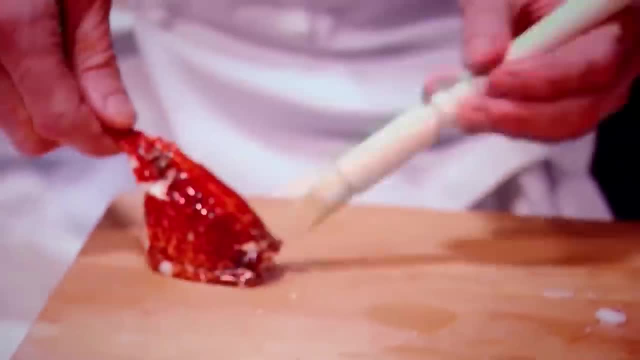 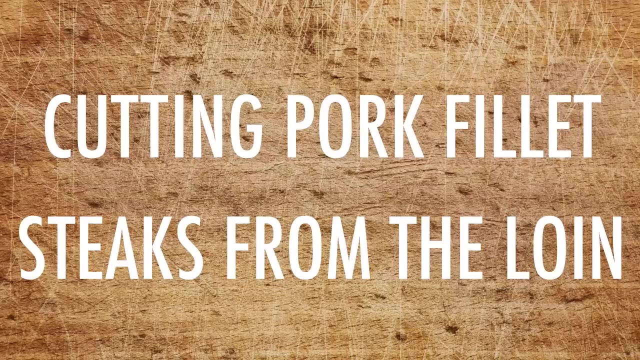 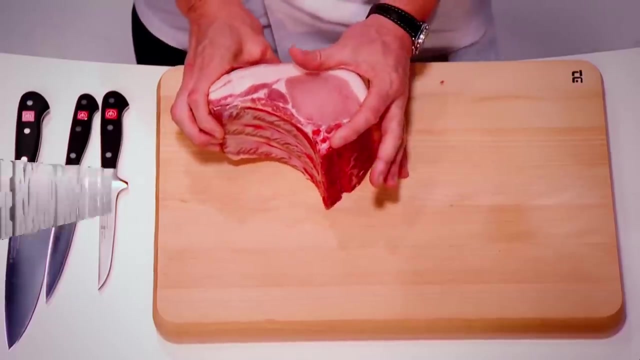 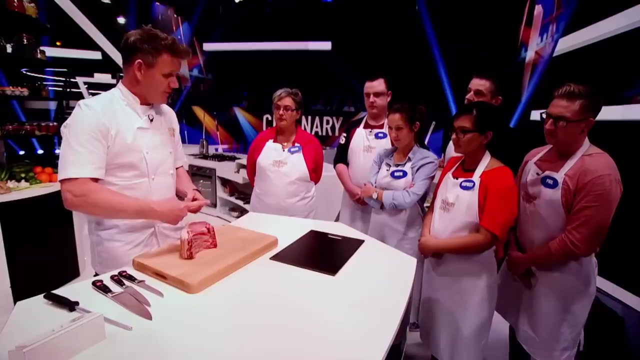 Brush the head, Touch of olive oil. That is how to extract your meat from your lobster Pork loin on the bone. The secret is now is to take that beautiful eye of meat off the bone and cut eight incredible steaks. First off, there's a T-shaped bone there. It's going through. There's the blade, There's the base. That there creates the most amazing crackling. 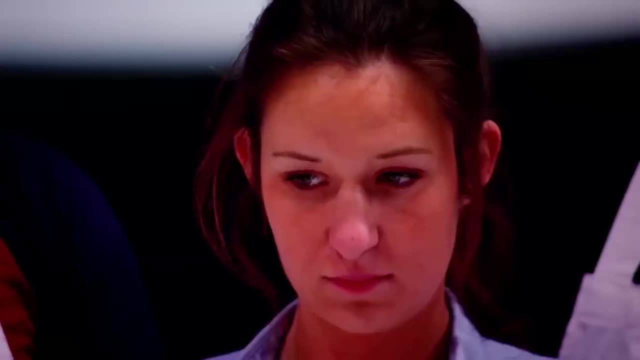 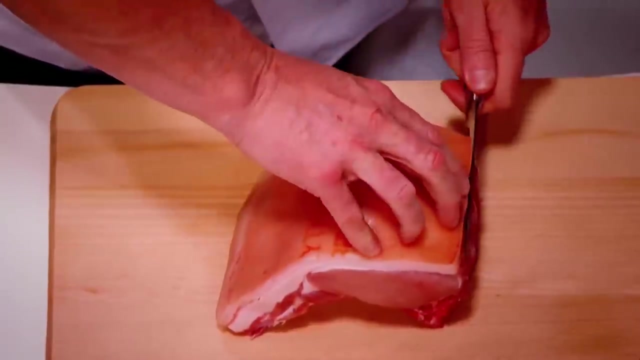 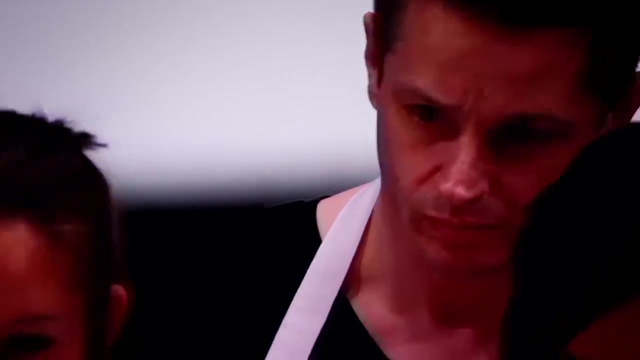 Make sure you stabilise Again. Boning knife: Super sharp, Really important. We're going to slice through there. Come down off the back, Slice throughand start to open up, Cutting In. There's a little ridge there. 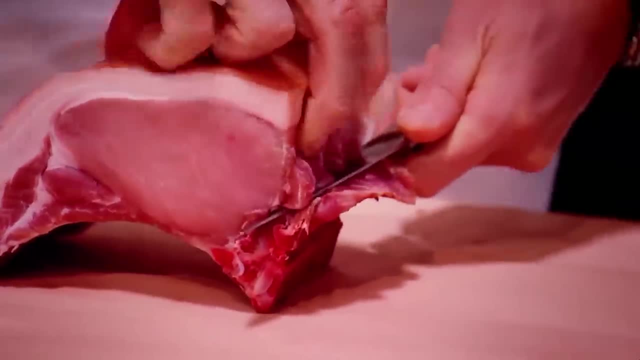 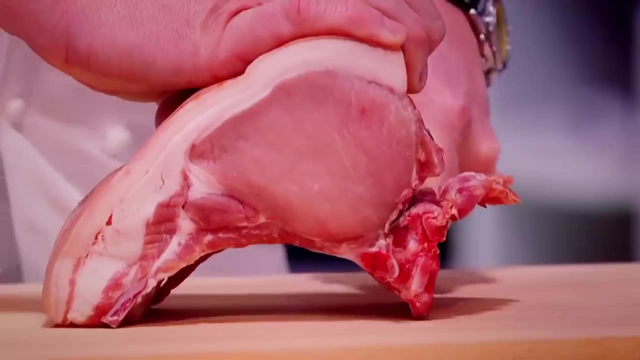 Come over the ridge, Careful not to slice through that. eye Fingers here Just pulling back. Once I start pulling back and I feel the lift off the loin of porkcome back down In Towards the bone, Then the next. 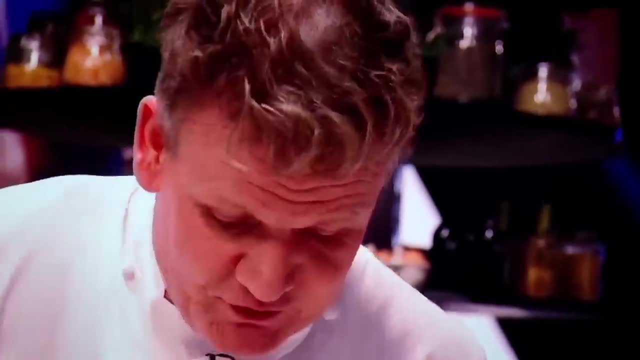 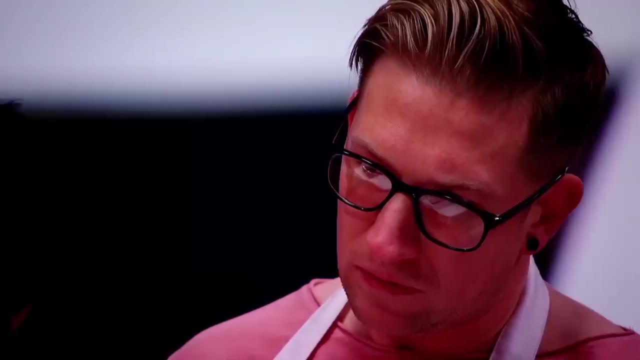 Turn the knife up into the eye of the meat You're going to destroy it Firmly, hold and slice down As you slice peel back. I want to see those ribs nice and clean Once we get there. this is a bendy, flexible knife. 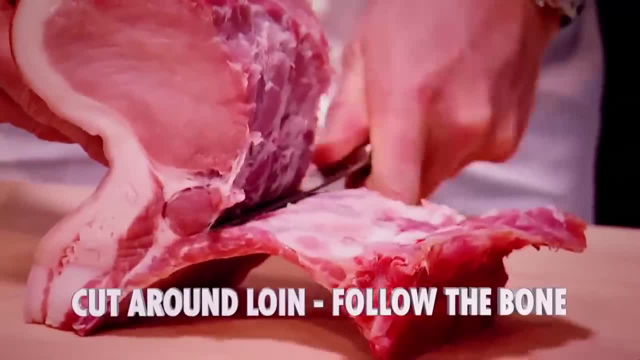 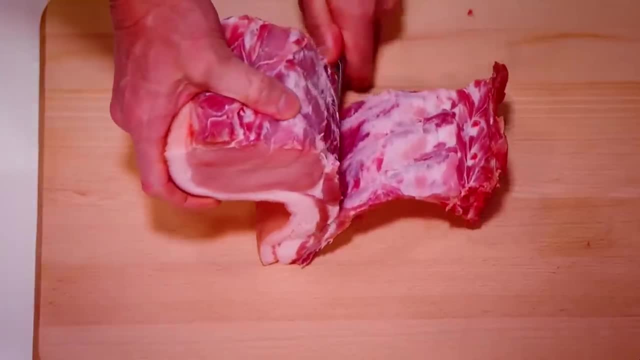 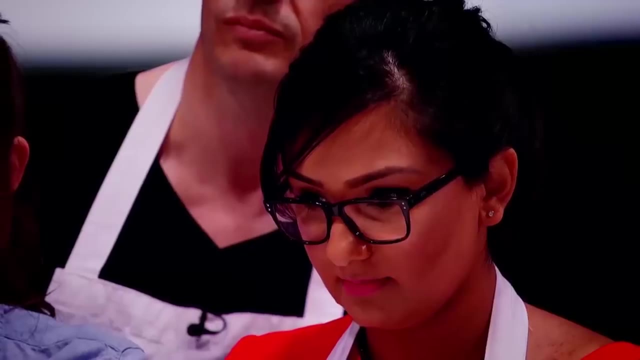 and it's done purposely for slicing. Follow the shape, Pull back, Look at where I am, Check what you're doing. Stay accurate, Stay close to the bone. Off Now loin bone. From there you can see the eye, the skin. 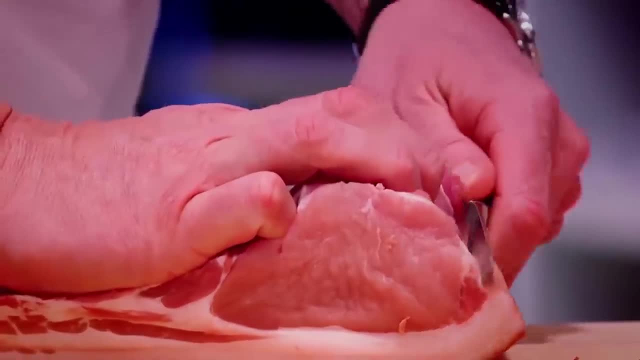 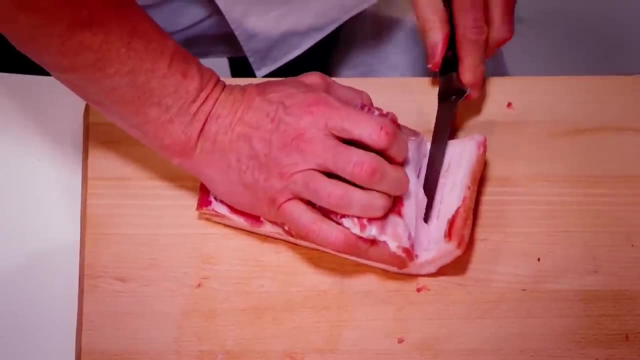 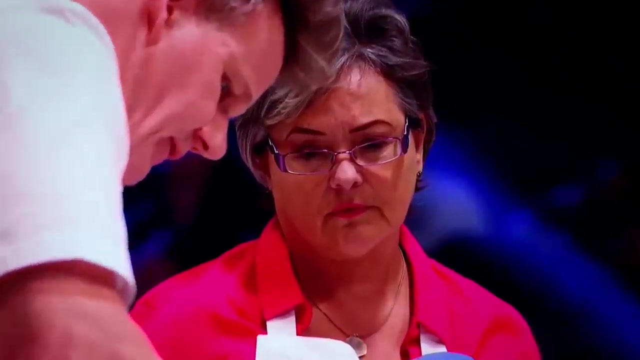 We turn it over flat side down, Come into the fat and we just pierce in there And then thumb inside, Nick, that little bit of fat through and literally pull off. Now look at the eye, Remove the arm. 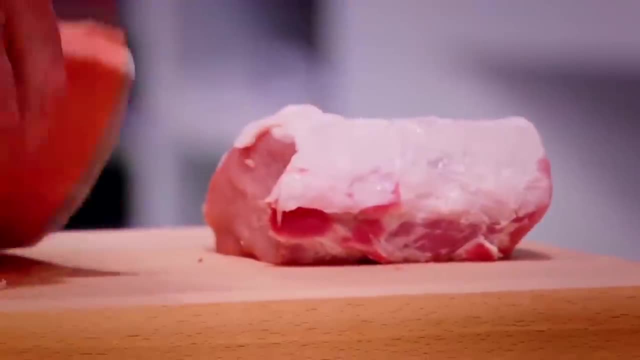 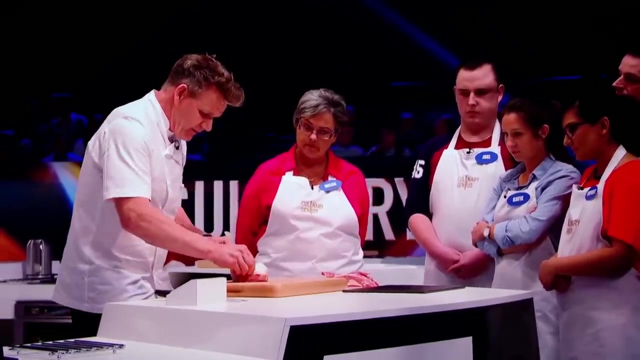 And then the other eye. That is the beautiful nut of meat That gets crispy. There's your crackling, From there the silver skin of fat. I want to go through the eye of the meat, but I want to trim this up. 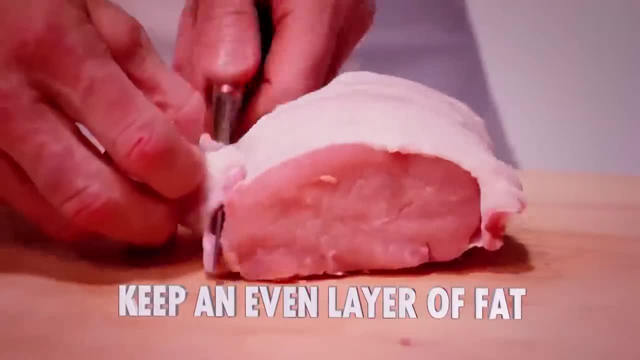 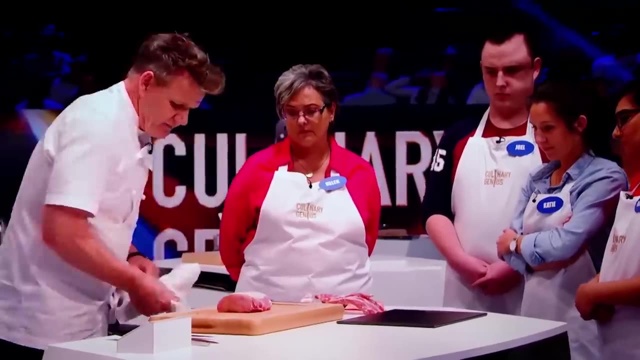 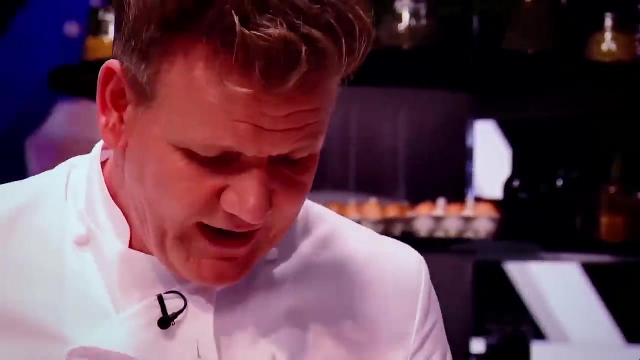 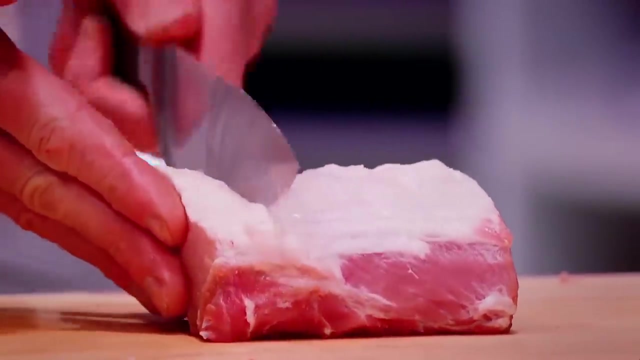 Pork is very lean so we have to leave a little cap of fat on there, Trim And then size up. We want four amazing cuts, Big knife for the weight. So it's four. so lightly mark there, there and there. 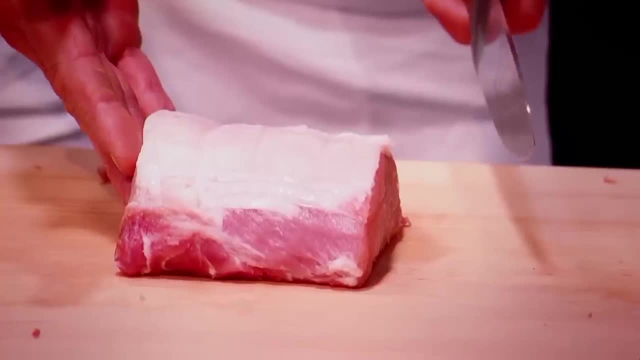 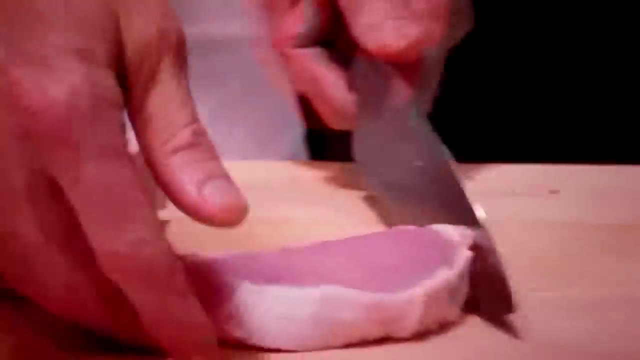 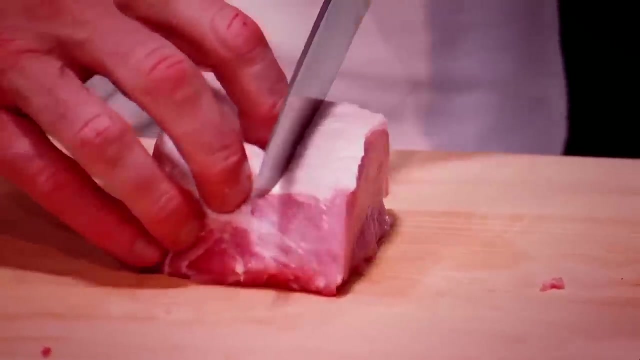 Pushing with this hand to keep that last slice super straight. Roll it up, Let the knife do the work. Slice down Off One beautiful loin of pork. Grip, Use five fingers. Grip, Stop the wobbling On. 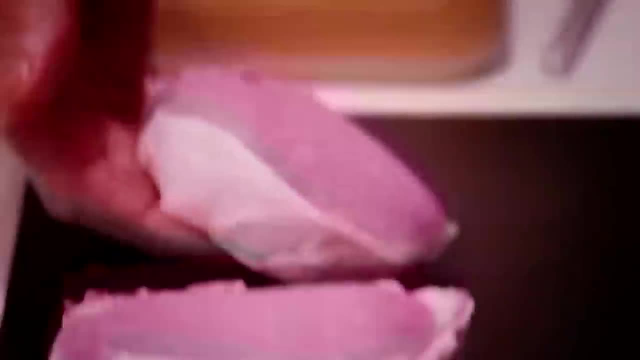 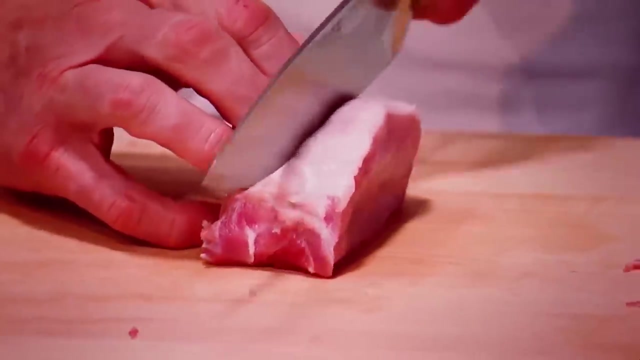 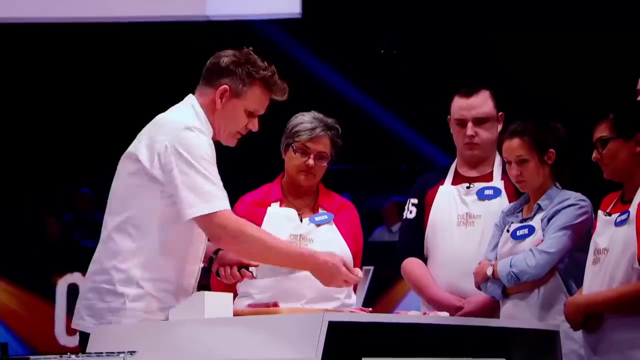 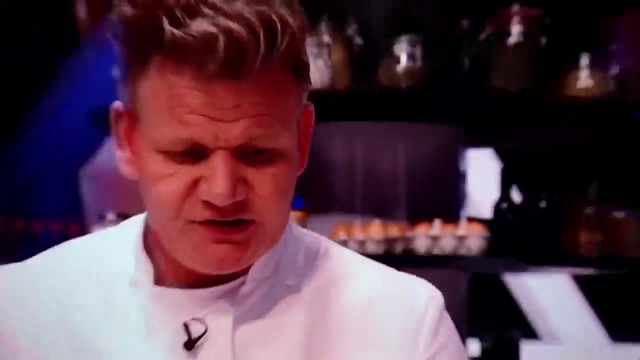 Hand on top, Let the knife do the work. Two Final, Size it up. Let the knife do the work. Open up the fingers there Come down Straight, Open And four. One, two, three, four, Stunning. 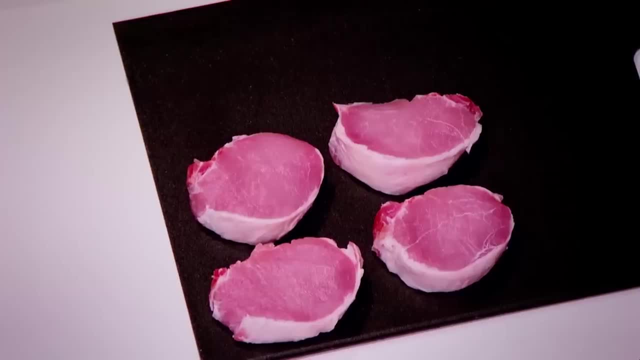 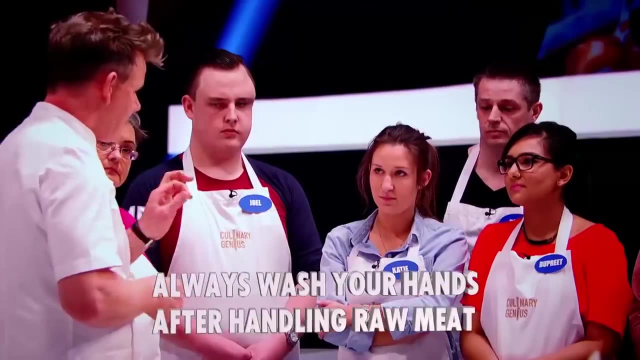 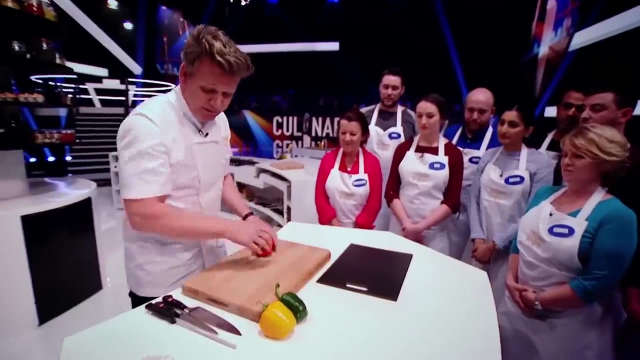 Loin Chops Off the bone. It's a great sear And literally six, seven minutes, Three minutes on each side. Let it rest. You've got pork at its best, Right, The most important thing when cutting peppers. 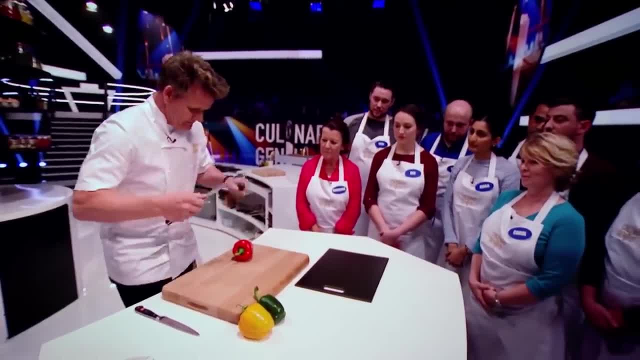 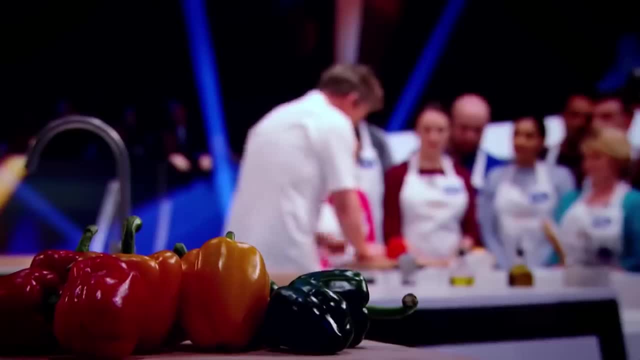 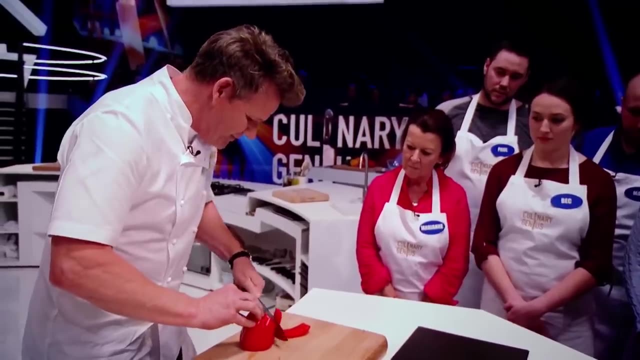 Secure the pepper, Okay, Make sure it's nice and stable. So first off, thinly, top and tail, Stand it up right, Clean the board every time And then Hold it up right, Slice round. Try not to go too deep into the seeds. 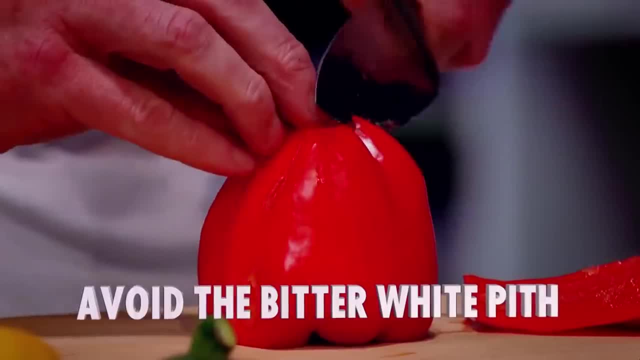 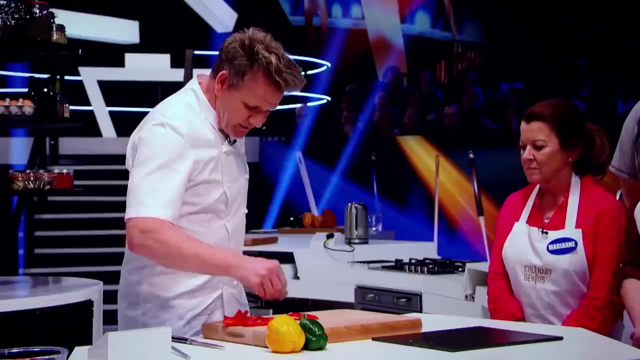 Okay, Otherwise we get that white part of the pepper off, And that's what turns it bitter. So keep the seeds intact. Now, from there, Straighten up your pepper, Use the board, Let the knife do the work, One finger in front. 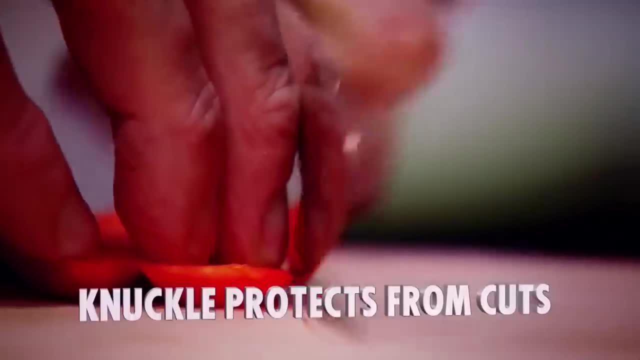 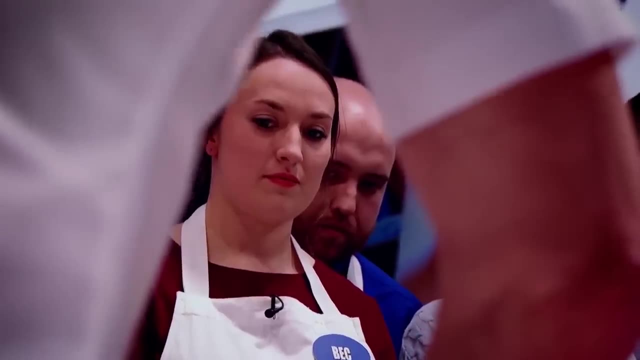 Two behind This knuckle protects the nail And slice nice and fine And fine. Let the knife do the work. Use the butt of the knife And slice those peppers nice and thinly. This is how you julienne the red pepper. 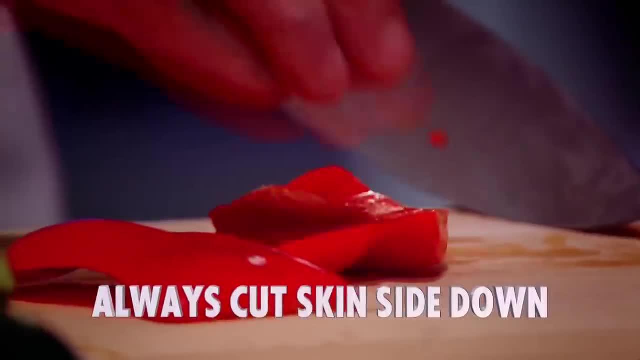 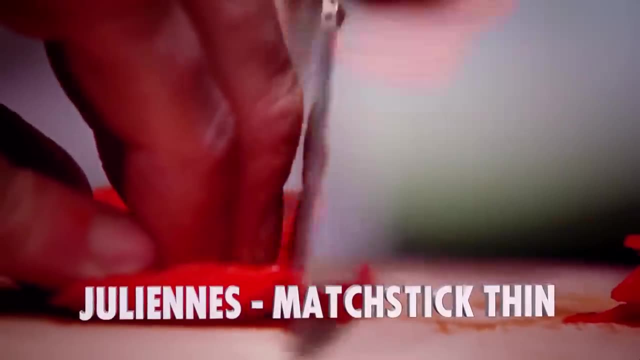 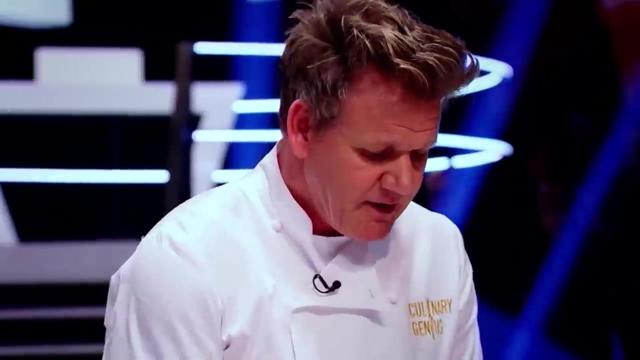 Always cut the pepper skin side down, Skin side up. Really difficult. Make sure those strokes are nice And thin. Thin peppers like this, Great for stir fries, Great for salads From there. Clear down. Next, Yellow pepper, Be a fine dice. 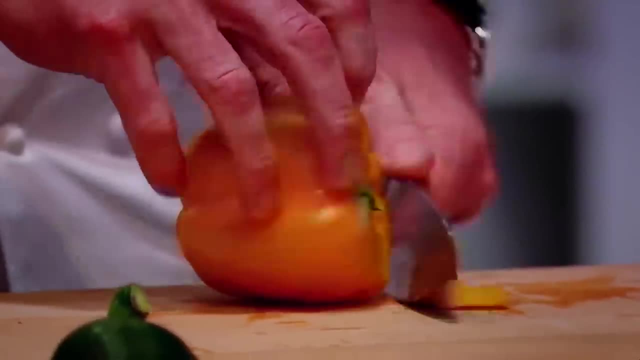 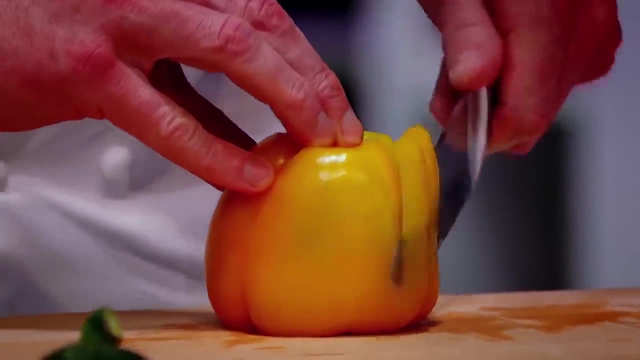 Similar way, Top and tail again. Literally secure the pepper Upright, Clean down. Follow the pepper coming around. Don't go too far into the center. Keep it nice and straight. Let the knife do the work. Keep the seeds intact. 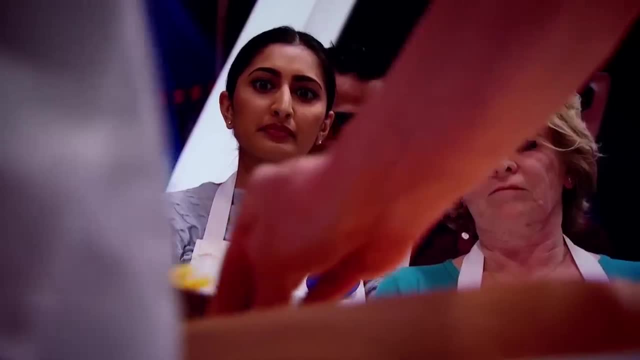 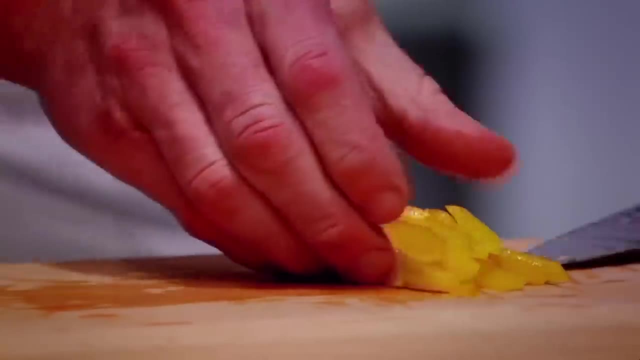 From there, Similar to the julienne Cut in matchsticks- All the way to the end. Don't worry about the speed, Be more precise. Clean the knife, Turn it around, Uniform them. Use your knife to uniform And then look. 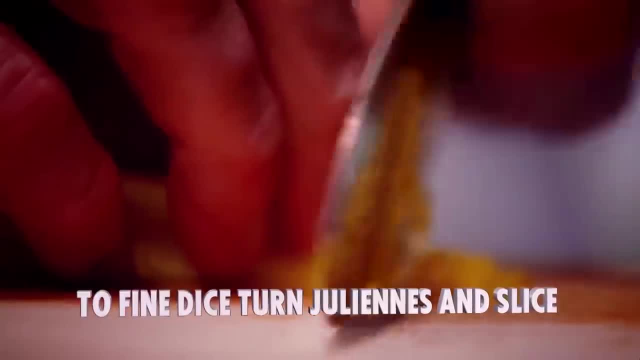 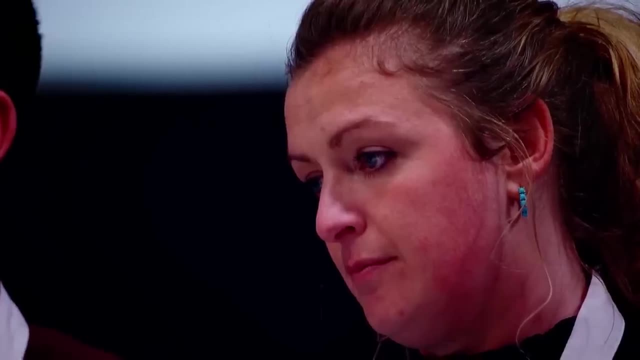 Up Nice and steady on the handle. Forget the speed That will come. Keep them nice and tight Like matchsticks. We've got that nice, fine dice All the way across. Lift up Onto your board Green peppers. 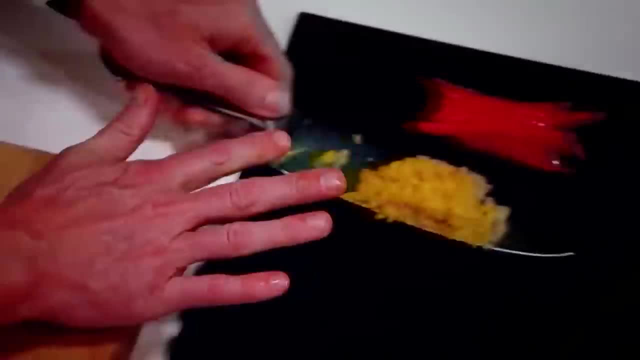 This one's going to be a baton, A bit thicker. Great for stir fries again And great for salads And great for sauces. Clean the board, Secure the pepper, Work around it, Make sure it's nice and straight. Don't go too far into the center. 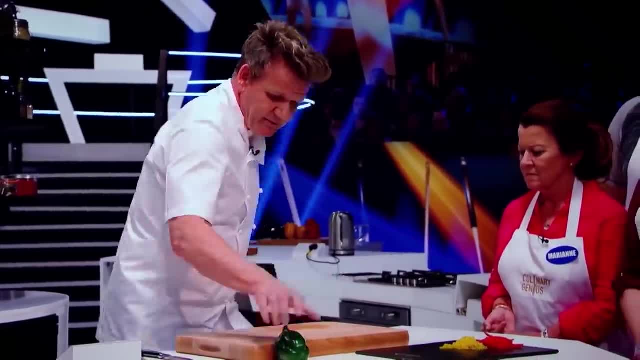 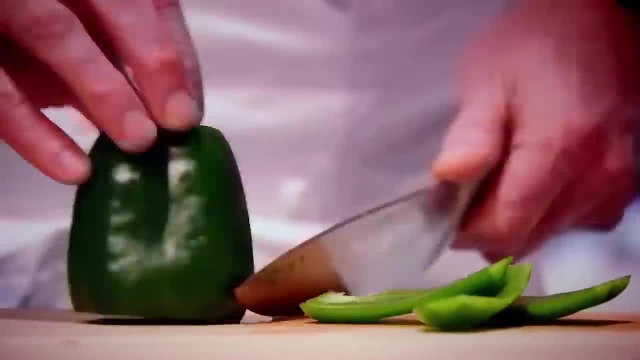 Keep it nice and straight. Don't go too far into the center. Keep it nice and straight. Don't go too far into the center. Keep it nice and straight. Secure the pepper, Work around And try not to take off any of that white stuff inside. 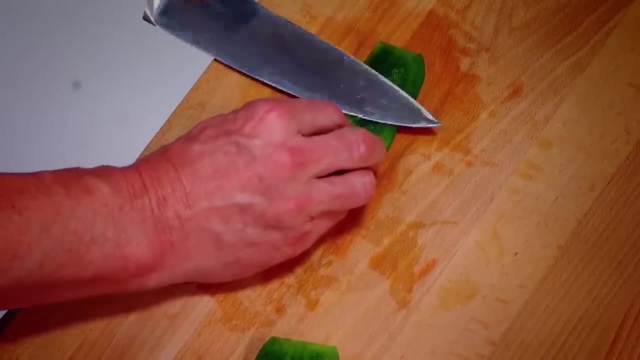 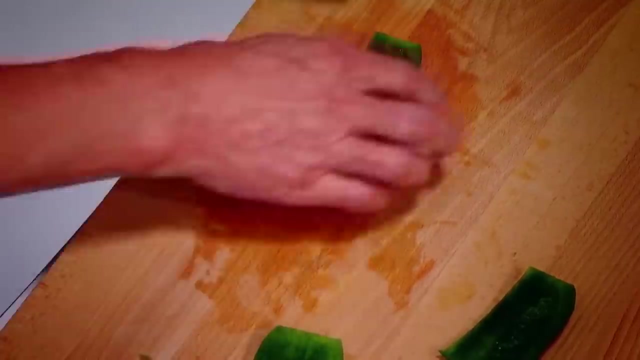 So look, I've got white on my pepper there. Hold it flat side down, Take the knife, Skin it off, Leave that on. You've got this bitter aftertaste on the pepper From there. square them up. Keep the knife nice and clean. 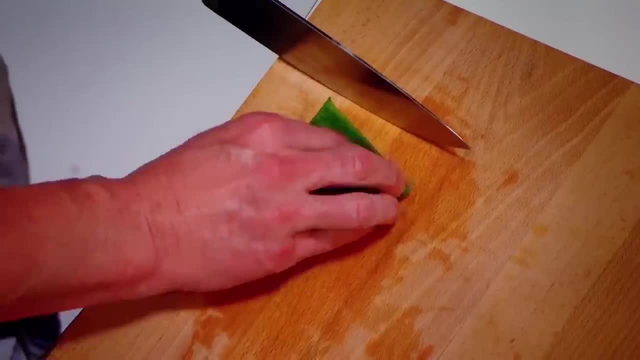 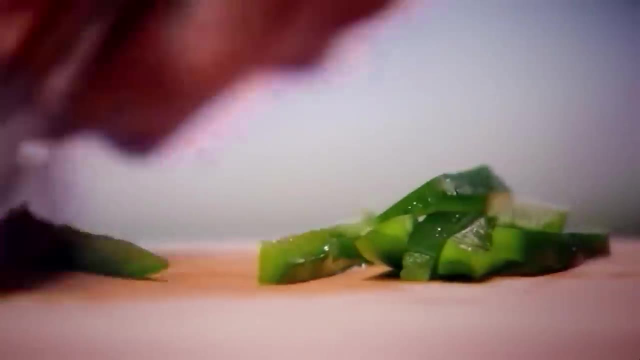 This time we go a bit thicker. So flatten the pepper down, And now we cut The most amazing baton. So we've gone from there, From a fine julienne, to a beautiful baton. Straighten the pepper out, Take off the little ends. 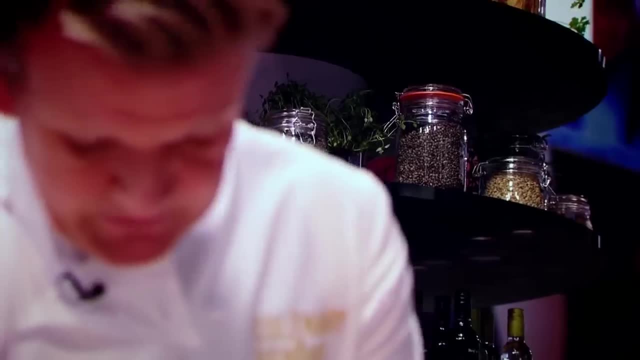 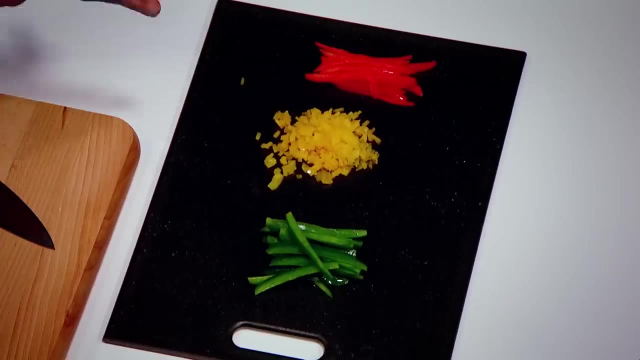 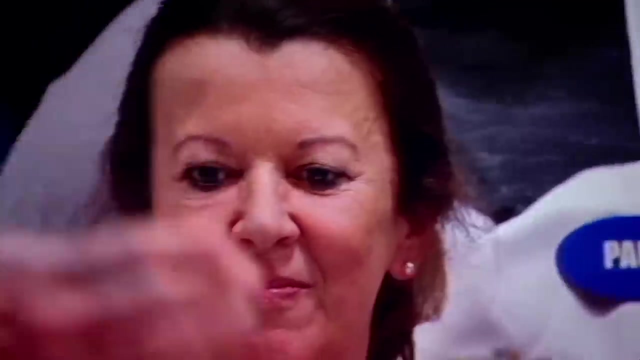 Nice thick slices And there we have a beautiful baton. Three peppers, three ways: Red pepper, julienne, Yellow pepper, beautifully diced. And this is how you baton the green pepper. Forget the rush, the speed, All about precision. 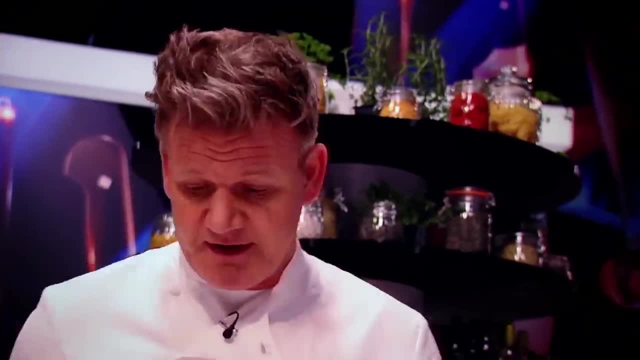 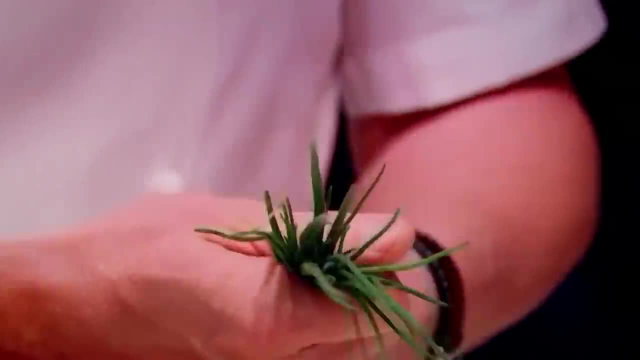 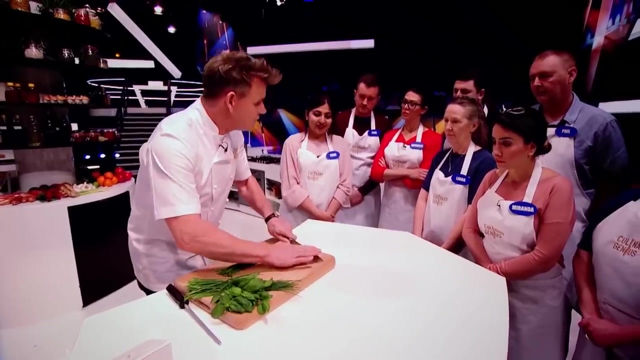 So first big challenge: chopping two herbs. very fine, Let's start off with the chives Secret here. keep that board clean, Stack the chives, These little tail ends discard. OK, How many times have you seen chefs chop? super fine. 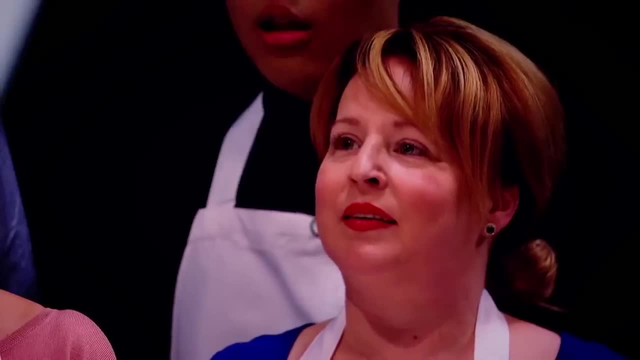 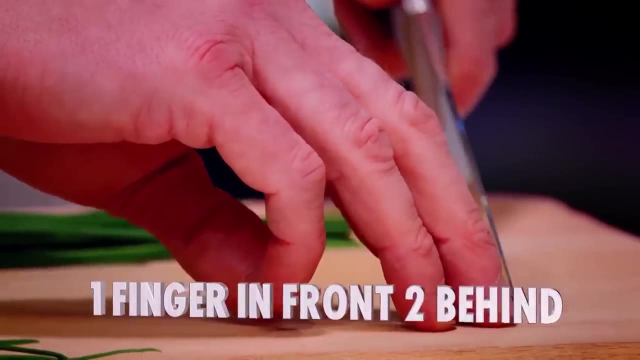 and the board's green. All the flavor's lost on the board. We want the flavor kept in the herb. So bunch up Three finger rule. One in front, two behind. This knuckle protects, Please be careful. One in front. 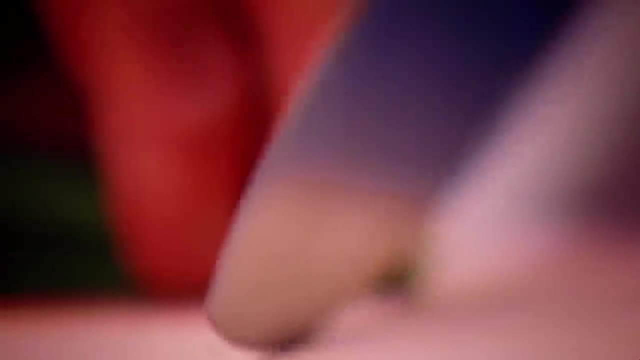 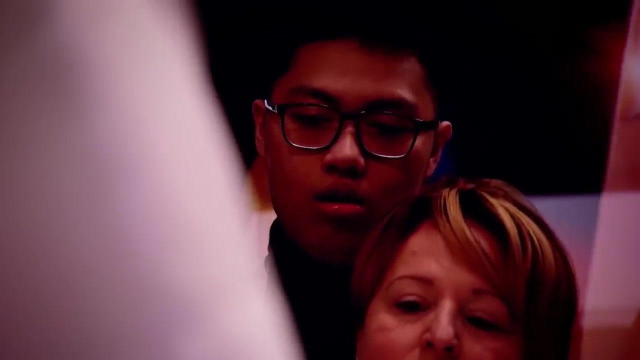 Let the knife do the work. Let's use the base of the knife And then literally just pinch. Nice and fine. They're called rundles because it's the shape of a round cylinder. Now stop, I clutch over the chives. 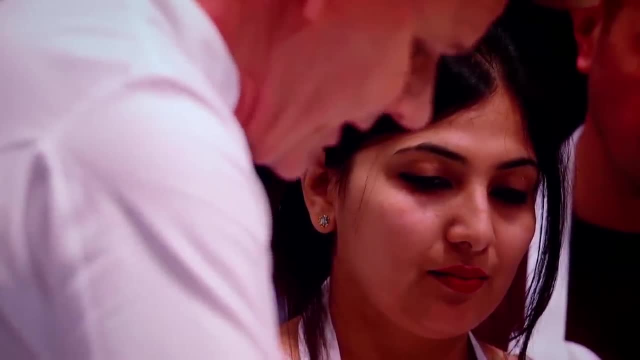 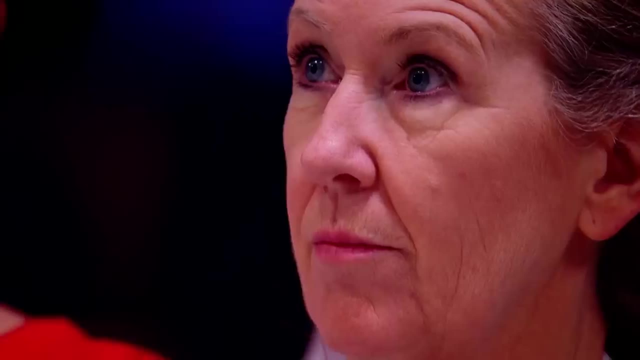 And I'm not pressurizing or bruising the chives So as we get the maximum flavor in the dish for the chives, I want the goodness of the chives in the dish, Not on the board, And look, No green on my board. 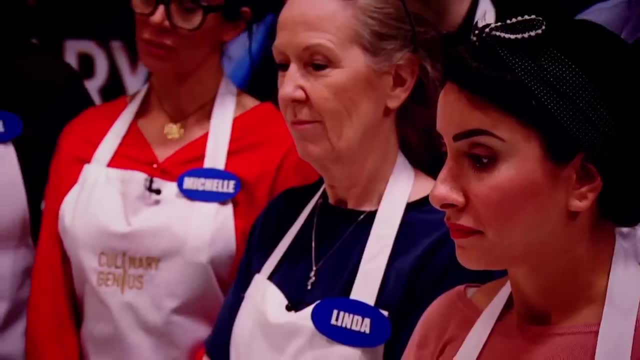 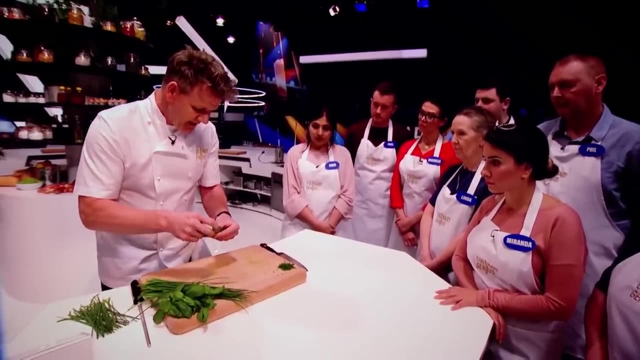 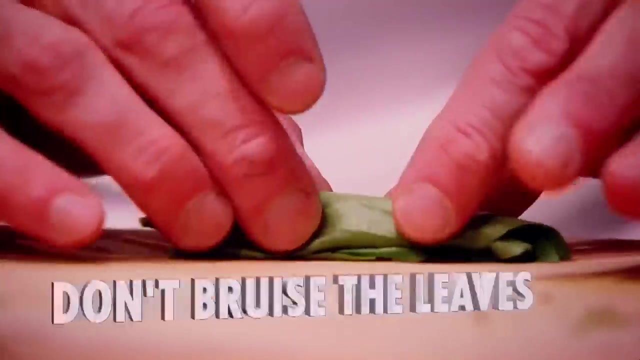 Super fine Chives. Come onto the basil. Open up the leaf. Tip to tip About 10, 12 leaves maximum, Otherwise it starts to bruise. Open up those leaves Gently, roll them Almost like a cigar. 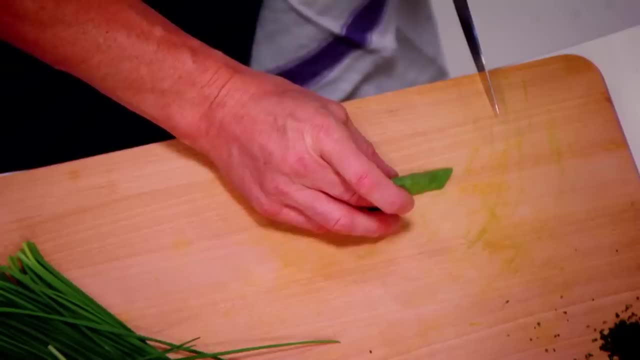 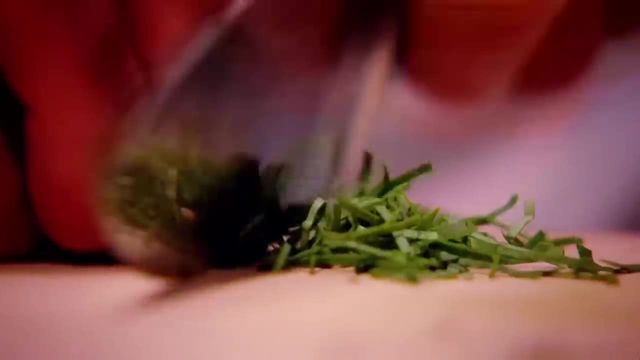 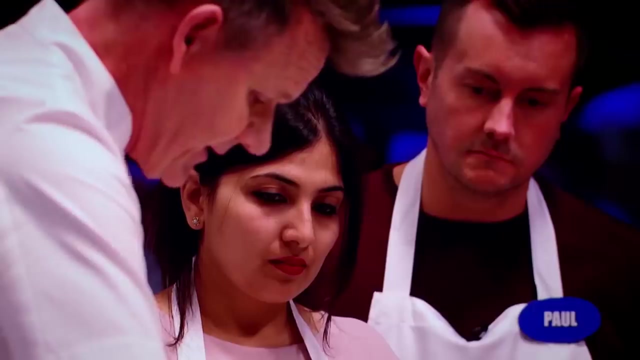 Don't bruise the leaf. Clean knife, Hold Finger Thumb, Three finger rule in front And again let the knife do the work. As you can see, the basil is not bruised, It's sliced super fine. In the culinary world this is called a chiffonade. 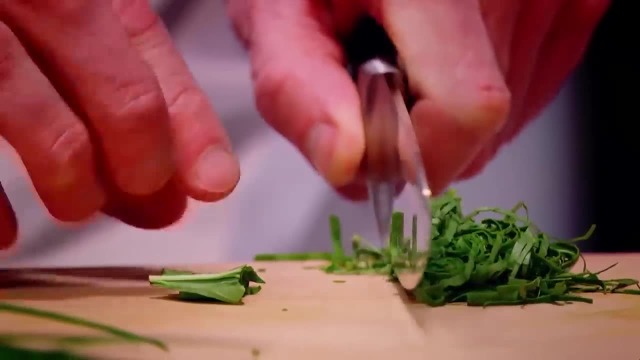 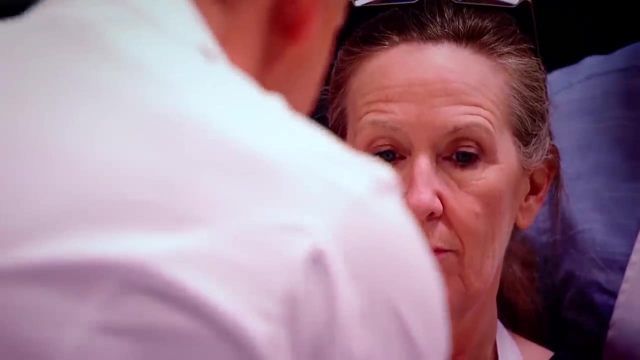 And it stays a beautiful color. If I had to push my fingers down and look what happens, The goodness comes out And there we have the most amazing chiffonade. Just smell that, The fragrance inside there. It's incredible And look. 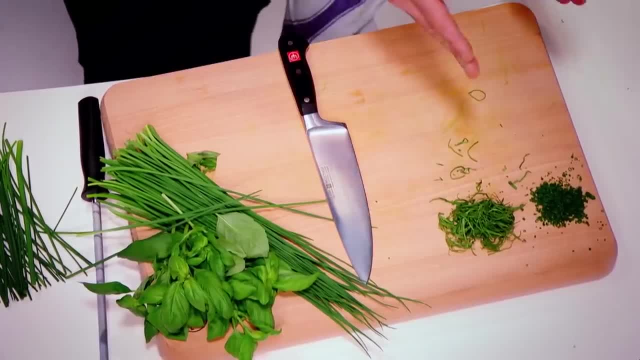 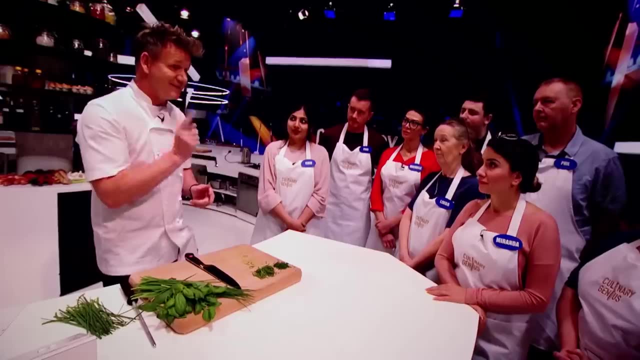 I've got nothing on my board: Clean, Super fine chopped chives And a super finely chopped basil. Both herbs chopped without bruising. There's a big difference. Understood, Yes.